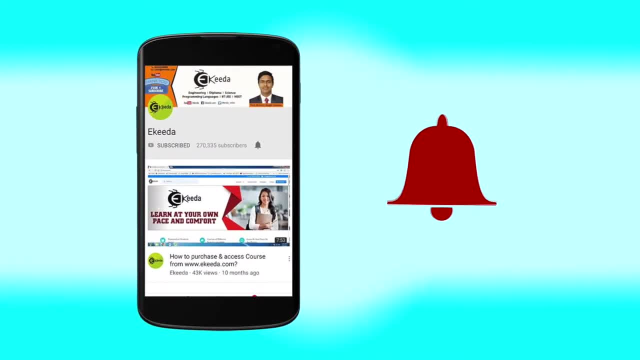 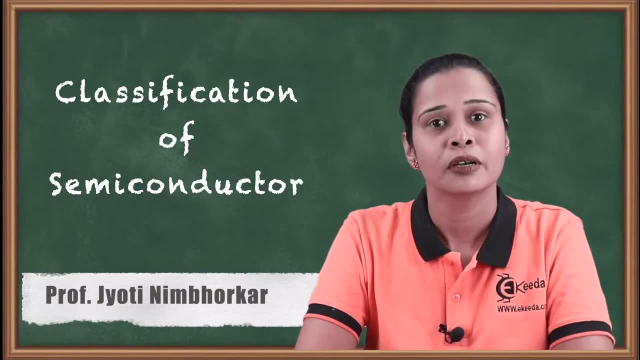 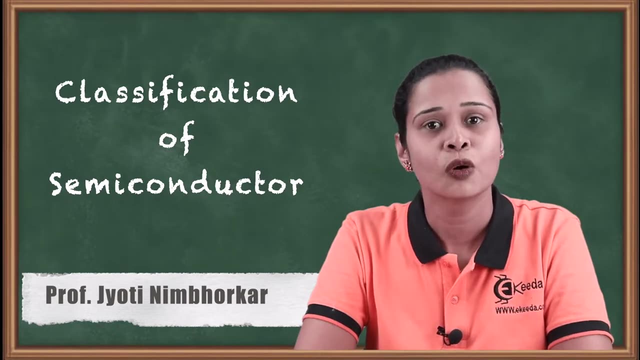 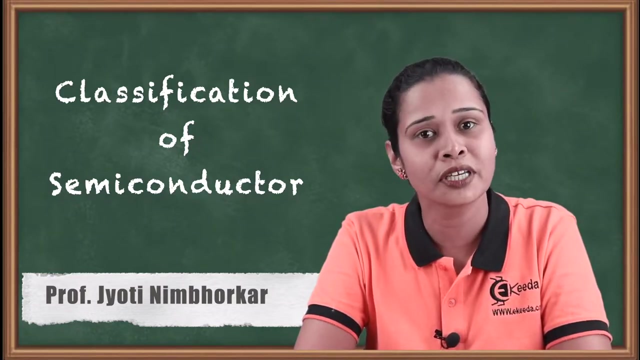 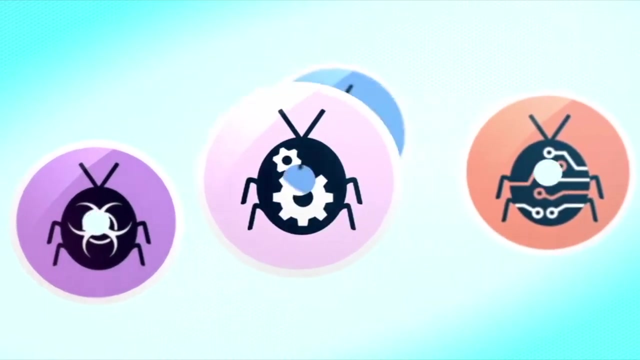 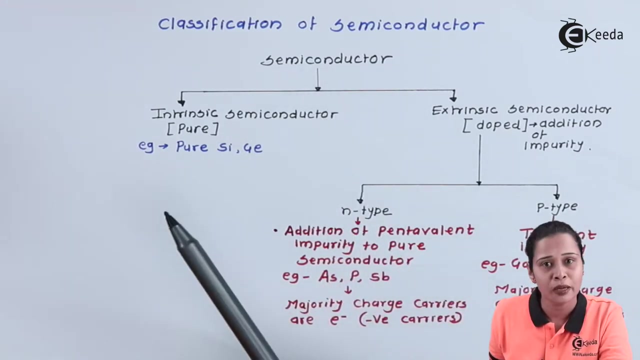 Click the bell icon to get latest videos from eKIDA. So let us see classification of Semiconductor Now, in classification of Semiconductor, we have two types of Semiconductor: Intrinsic Semiconductor and Extrinsic Semiconductor. Intrinsic Semiconductor is a purest form of Semiconductor. 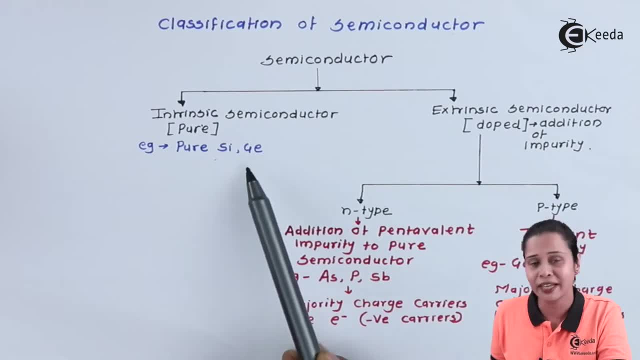 The example of Intrinsic Semiconductor is Silicon and Germanium, But getting Intrinsic Semiconductor is quite difficult because it is a purest form and purest form material we are getting that is rarely So. the process of getting or extracting pure Semiconductor is quite costly. 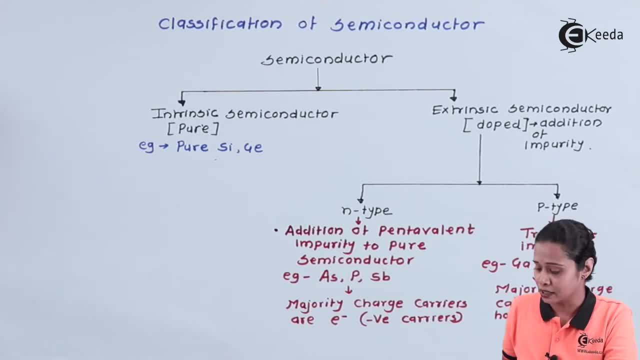 But we have two type of pure Semiconductor, that is, Silicon and Germanium. The second Semiconductor, the type that is Extrinsic Semiconductor, This is also called as Doped Semiconductor- Doping, it is a process of addition of impurity. So here we are adding two type of impurity. 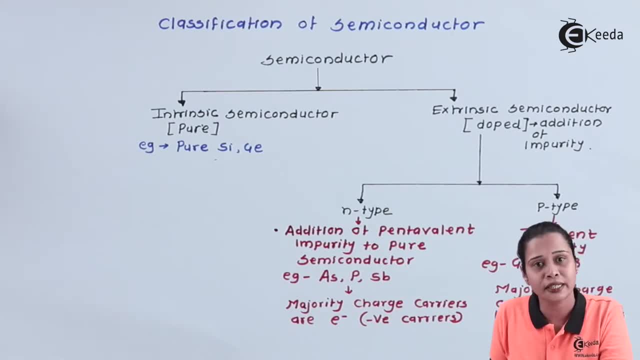 The first one, that is Pentavalent impurity, and the second one, that is a Trivalent impurity. So if we are adding Pentavalent impurity, then this Semiconductor is called as N-type Semiconductor, And if we are adding Trivalent impurity, that Semiconductor is called as Intrinsic Semiconductor. 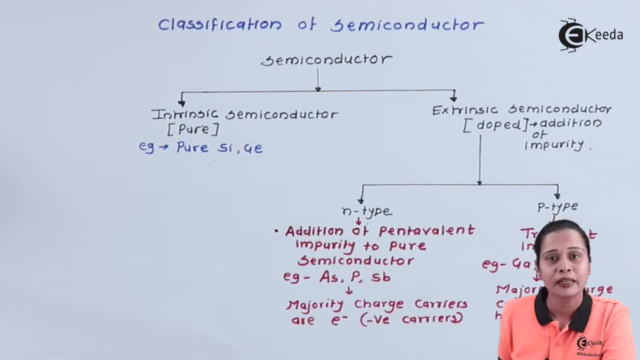 It is called as P-type Semiconductor. Let us see what happens in case of N-type Semiconductor. So in N-type Semiconductor we are having Pentavalent impurity. Pentavalent impurity means there are five valence electron. Valence electron means the electron which is present in the outermost cell. 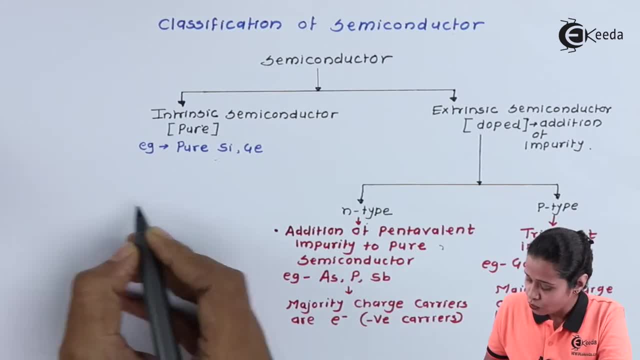 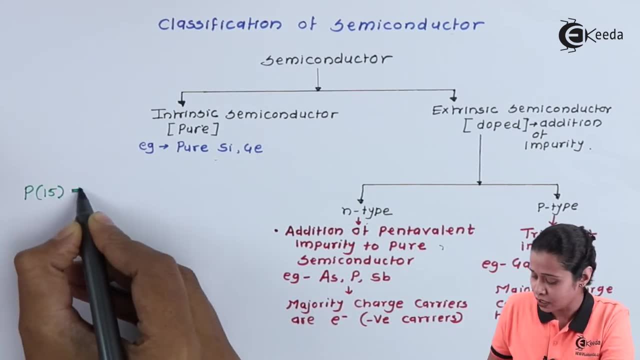 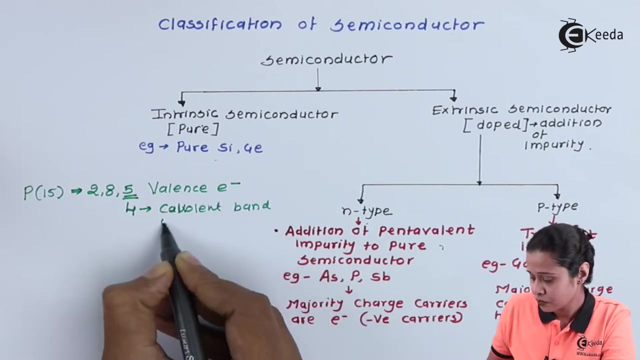 For example, suppose we are taking a Phosphorus. So Phosphorus P And its atomic number Atomic number is 15.. So here we have 2,, 8 and 5. So there are 5 valence electron. Now out of this 5 valence electron, 4 electron will make covalent bond with silicon atom. 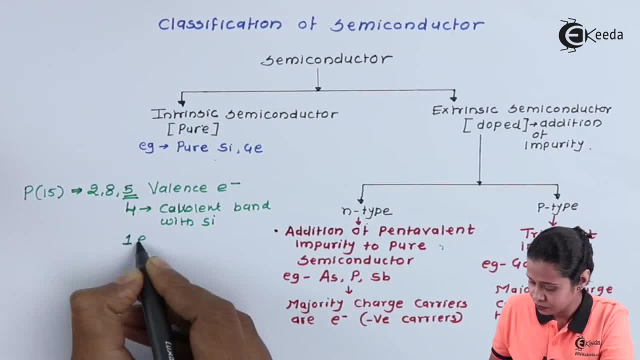 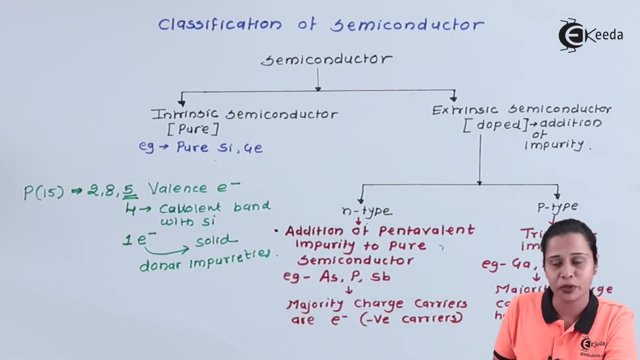 And still there is one extra electron. So that electron we are donating to the crystal or solid, or we can say to the Semiconductor, So we are donating that. So this pentavalent impurity is also called as Donor impurity. These are Donor impurities. 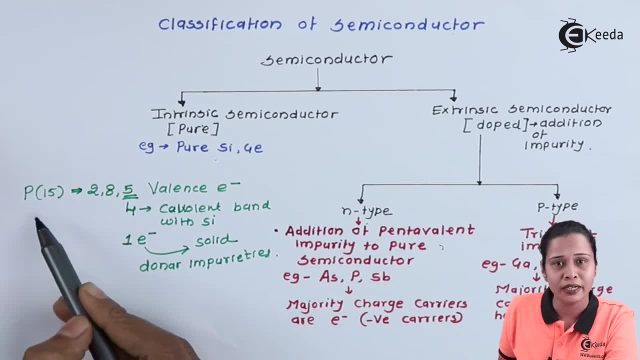 Now, in this case we have so many pentavalent impurities, Means in the solid We have so many pentavalent impurities, So many valence electrons. So In a solid we have such a n number of electrons. That is donor electron. 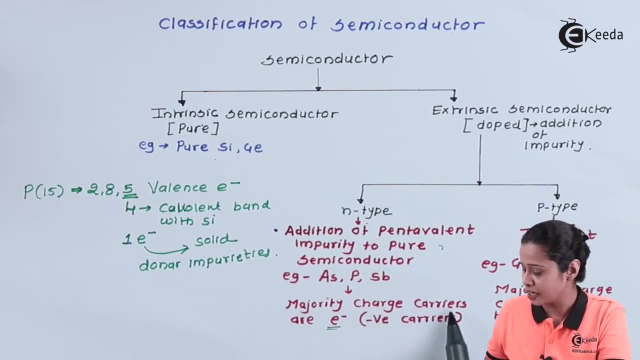 So Because of this we can say the majority charge carriers In case of n type impurity Or n type Semiconductor. It's a electrons, So there is a current conduction in n type Semiconductor. Hence the current conduction in n type semiconductor is due to the electron and that 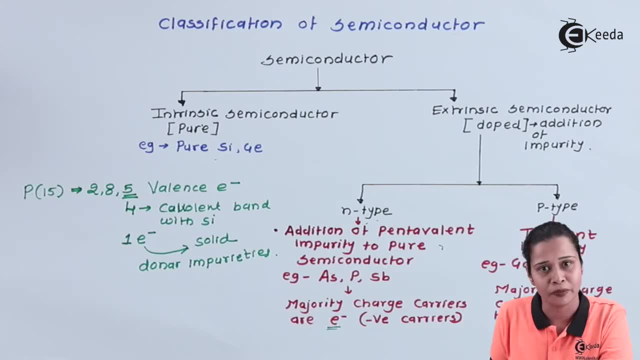 electron we are getting from the pentavalent impurity. As we know, the electron is having a negative charge, So these are the negative charge carrier and that negative stands for n. That's where this semiconductor is called as n type semiconductor. Let us see what is p type. 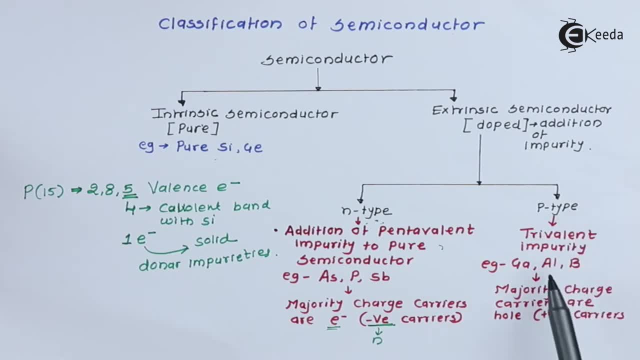 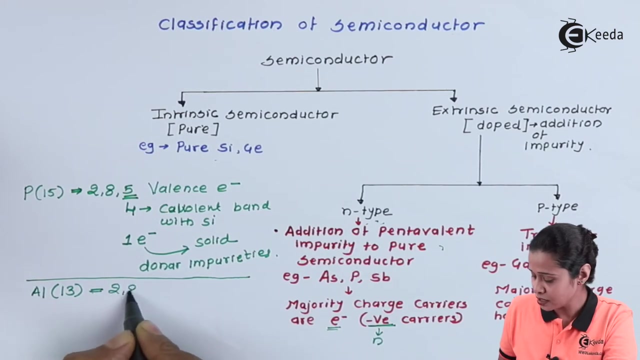 semiconductor. In case of p type semiconductor, we are adding trivalent impurity. Trivalent means in outermost orbit. there are three valence electron. Just take an example of aluminium. In case of aluminium, its atomic number is 13.. So configuration is 2,, 8 and 3.. 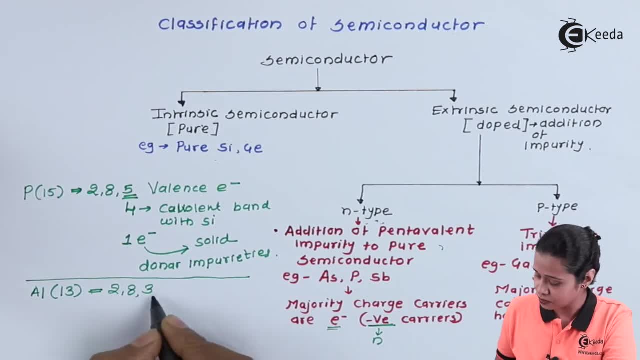 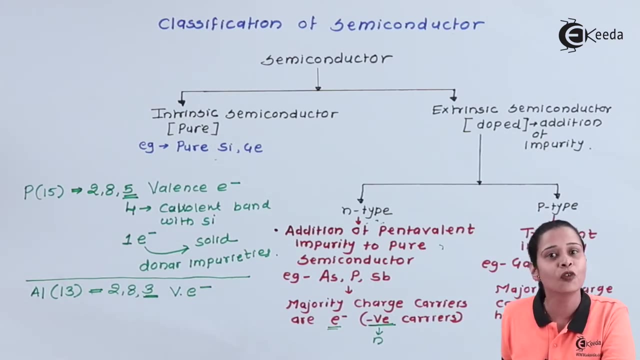 So here we have three valence electron. These are the valence electron. So in trivalent impurity we have three valence electron, This three valence electron making a covalent bond with the four silicon atom, that is, with the neighboring silicon atom. So in this case we have four silicon. 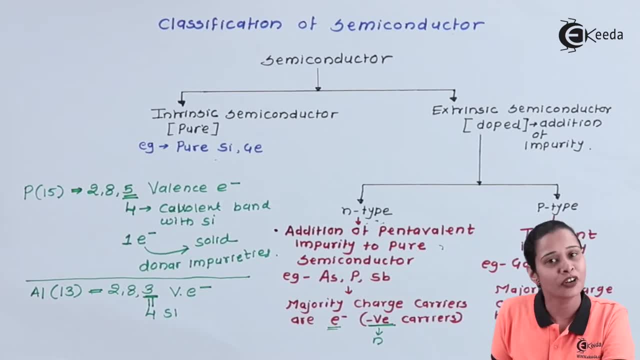 So this three valence electron of trivalent impurity make covalent bond with the four neighboring silicon atom. Now in this case we will see we have a four silicon atom, but here in trivalent impurity we have three valence electron, means one covalent bond will remain. 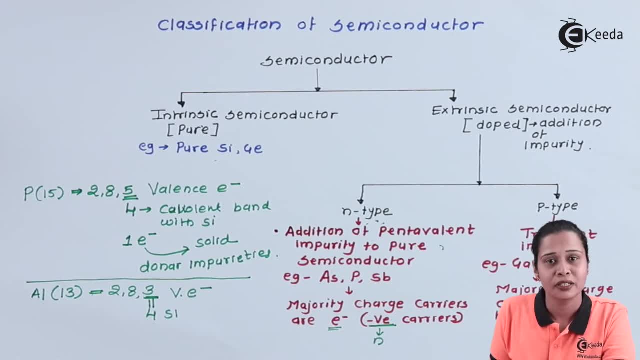 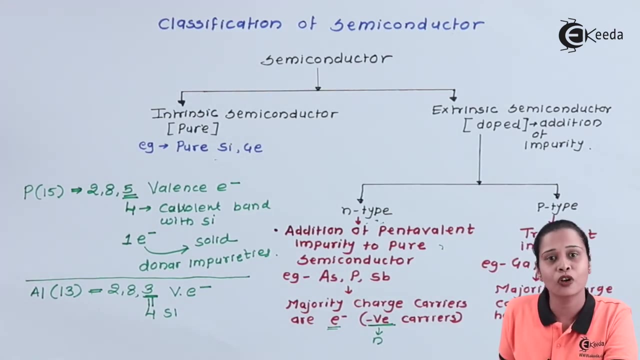 empty. That empty position is called as hole. So if we define hole then we can say hole is absence of electron in the covalent bonding, So it consists of the vacancy for the electron. or we can say it is ready to accept electron. that's why this impurity is called as acceptor. 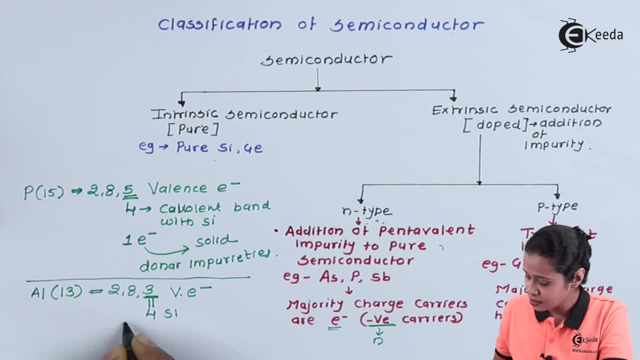 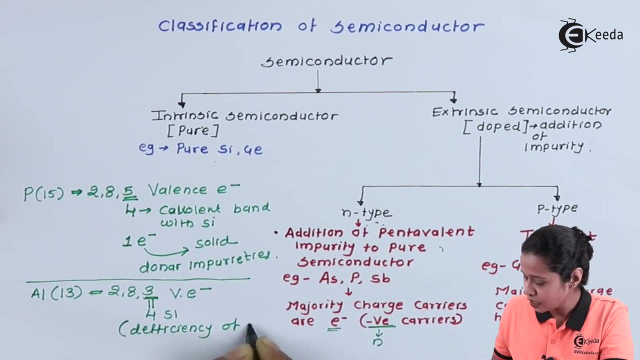 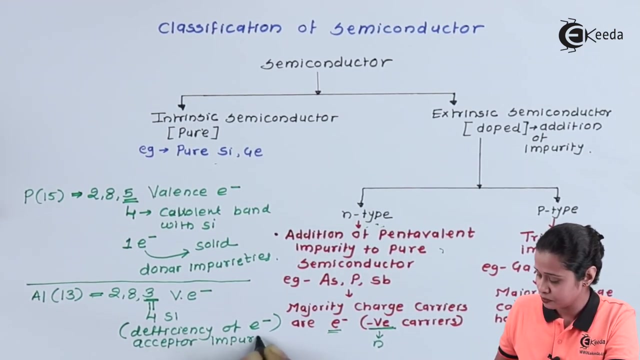 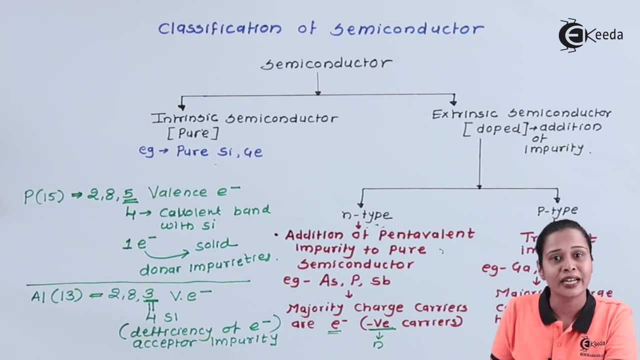 impurity There is a deficiency of electron means that material is ready to accept electron. that's why this impurity is called as acceptor impurity. Now, in this case, we have a absence of electron. that is a hole, and that hole is having virtual 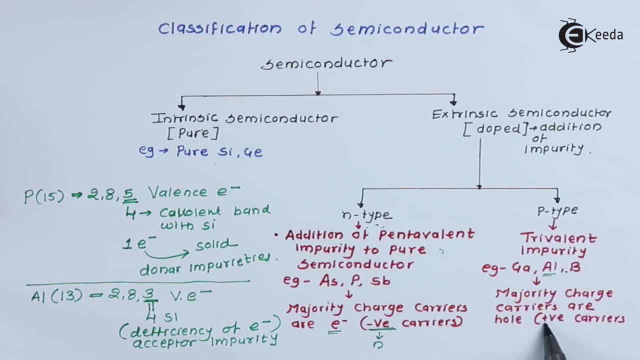 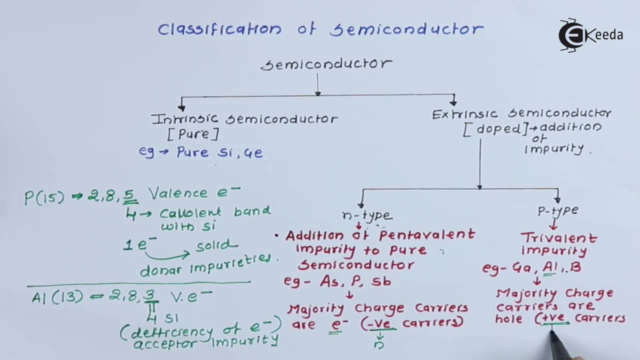 positive charge means. here we are seeing the charge carriers here, that is, majority charge carriers are positive carriers, so that positive stands for p. hence this material is called as p-type material, so in this way we can classify semiconductor. Thanks for watching this video. stay tuned with eKIDA and please subscribe eKIDA. you.